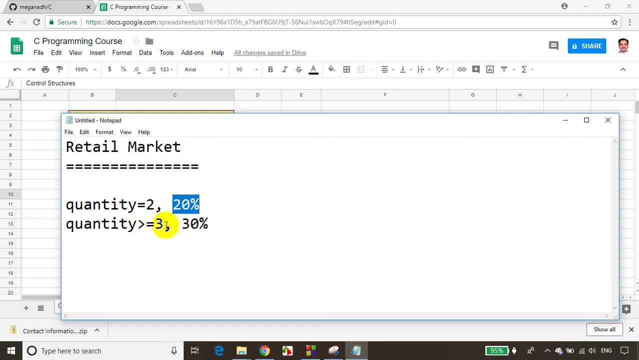 you need to write logic with the 20% discount. If quantity is greater than or equal to 3, you need to provide logic of 30%. Now, this kinds of decision making will help to skip some statements or join the logic based on the condition. So these conditional statements are repetitive statements or we have categorized into control structures. Now let's try to have a look at this list of control structures before we jump into write some examples. Right? So let's see this now, We'll see this. 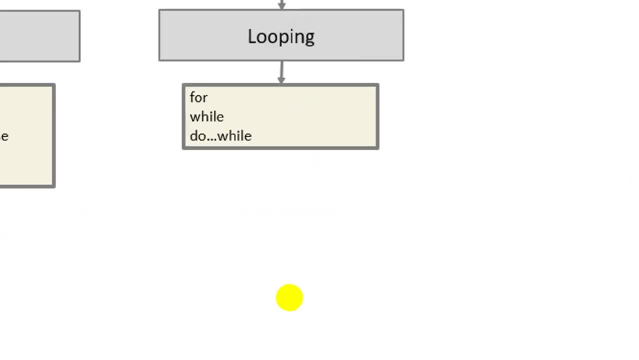 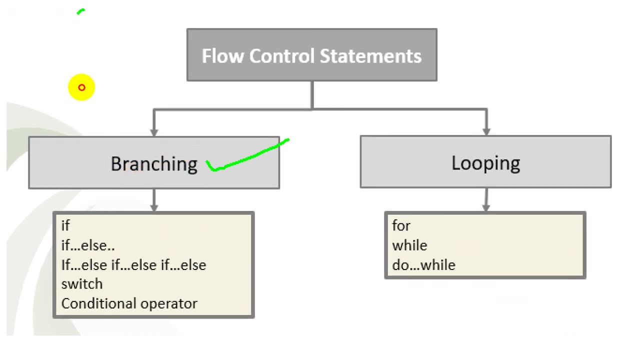 the list of control structures. now you can see here control structures or flow control structures are categorized into two types. one is branching. so branching is basically like, based on a condition, take a decision in which flow you want, to which direction you want to go ahead. so if condition 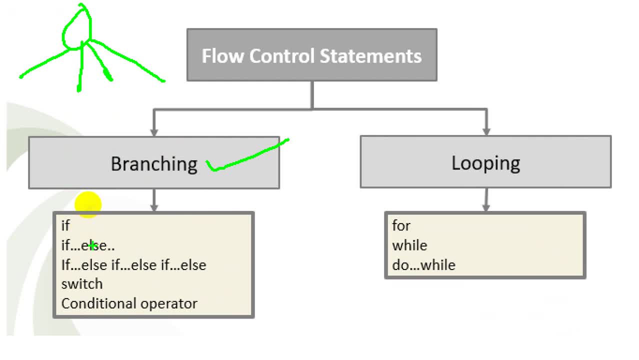 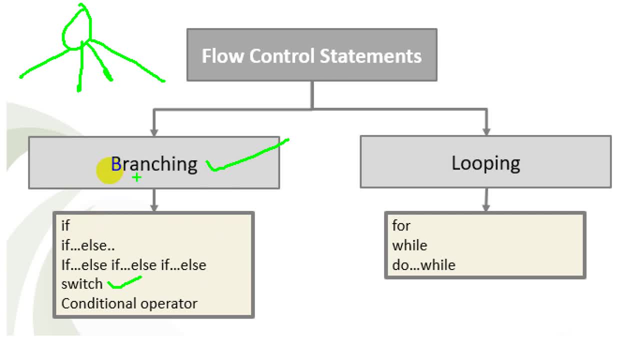 also used for branching, where one condition you need to execute when you have like multiple options. so, based on, based on the condition, based on the user selection, you want to execute only one statement from. let's take 10 statements, so you'll go for switch case and we'll also see about conditional operator, how, if else, can be written in single line using: 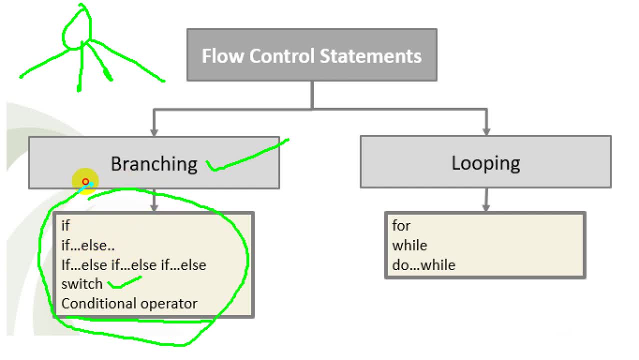 conditional operator. so all these comes under branching, because the code flow happens based on the condition one. one of the statements get executed. now coming back to looping, let's take you want to do some repetitive tasks, so you want to print hello five times so you can use a for. 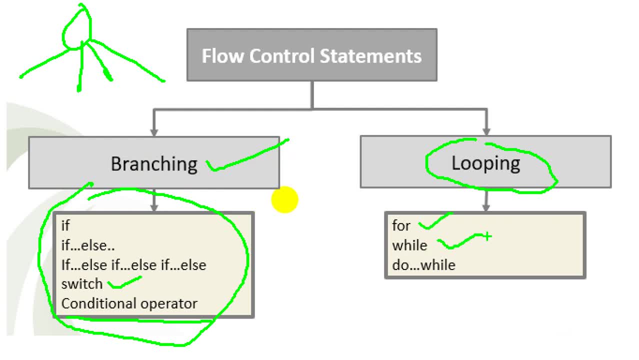 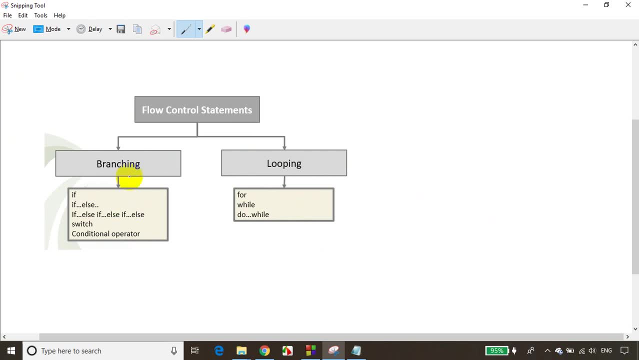 loop to print five times. you can use a while loop to print hello five times, so and a do while loop, so for loop while loop. and do while loop, so you can use a for loop to print hello five times. do while loop are categorized into looping and we'll see some examples and where exactly we can. 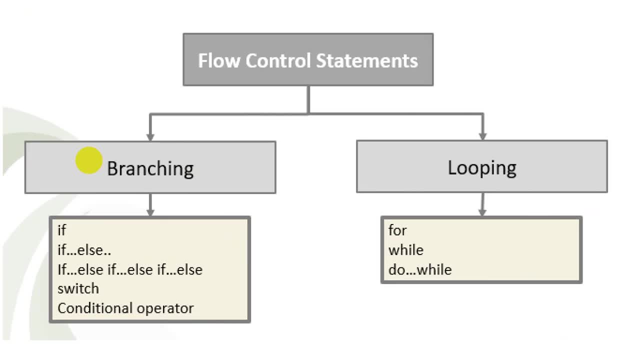 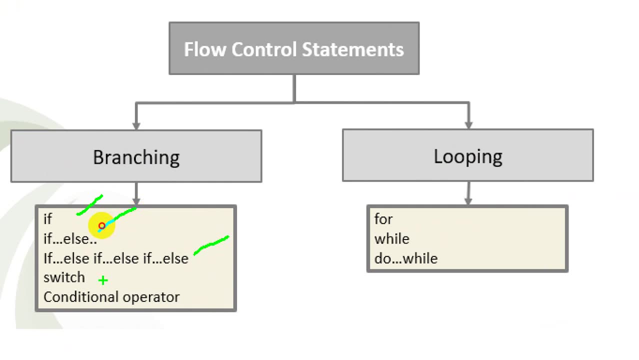 use them in real world projects. so so control structures are categorized into branching and looping, and branching we have if, if else, if else, if else, if l statement and switch case and conditional operator. so we'll see that in detail in the next module. and looping is for loop, while loop and do.